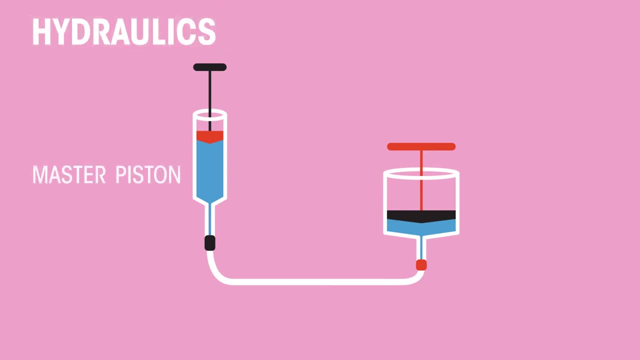 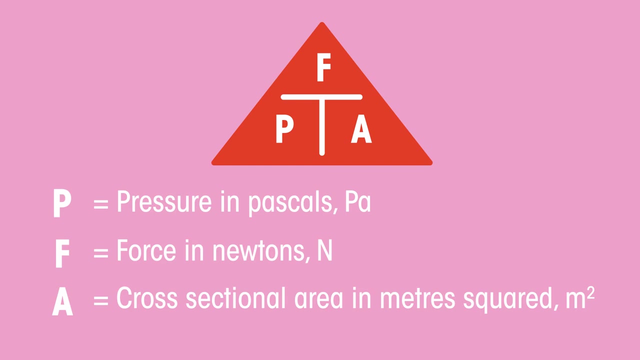 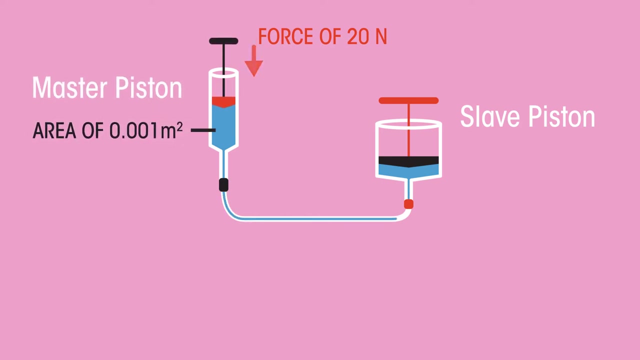 Hydraulic systems consist of two pistons: A master piston, where pressure is applied, and a slave piston which the pressure is transmitted to. Let's look at an example of how system multiplies pressure. Remember pressure is calculated using this equation: A force of 20 Newtons is applied to the master piston, which has an area of 0.001m2.. 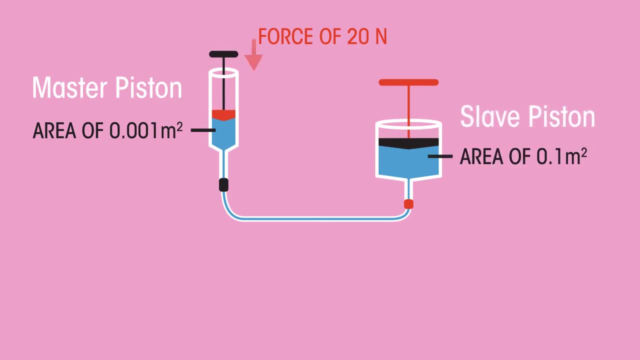 The slave piston has a surface area of 0.1m2.. What force is produced by the slave piston? First we need to calculate the pressure produced by the master piston, So 20 Newtons divided by 0.001m2 to give 20,000 Pascals. 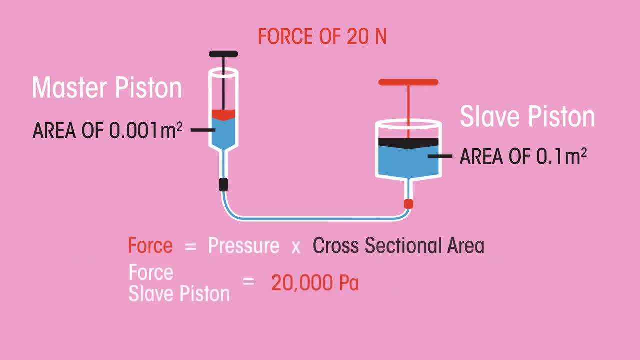 Now we need to calculate the force produced by the slave piston. So 20,000 times 0.1m2 to give 2,000 Newtons. So the force on the master piston was 20 Newtons, but the force applied to the slave piston. 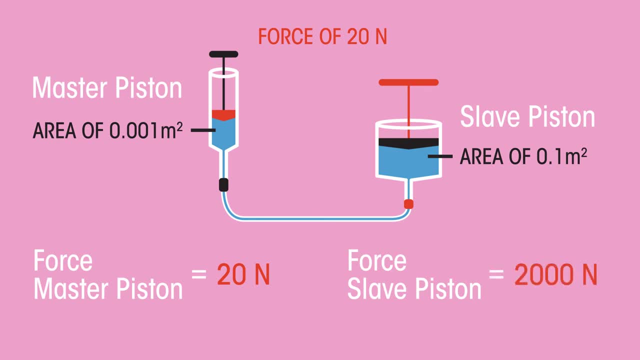 was 2,000 Newtons. The force has been multiplied. Small force on a small area has resulted in a much larger force on the slave piston. It's the same principle that is used in hydraulics: A small input force has resulted in a 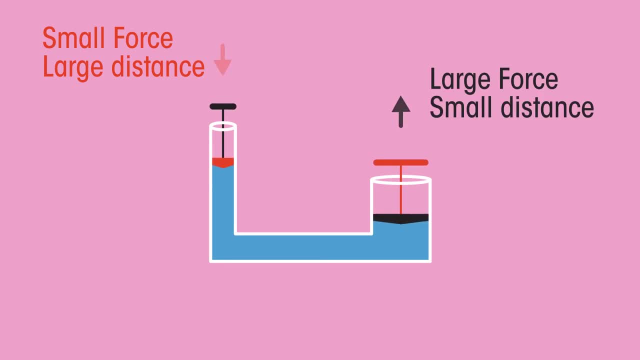 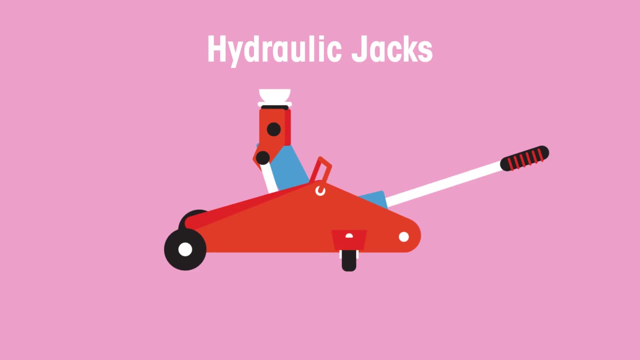 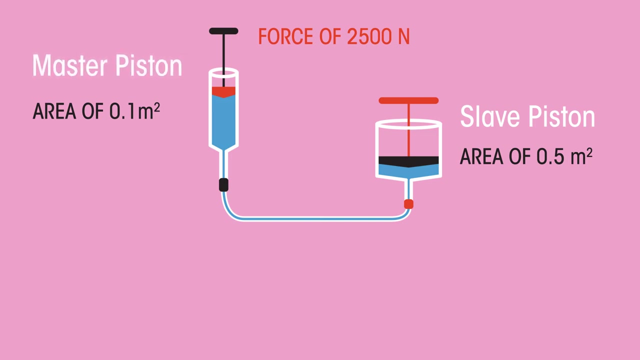 large upward force. Exactly this, but on a much larger scale, is used to generate forces strong enough to lift things like hydraulic jacks. Now it's your turn to try an example. A force of 2,500 Newtons is applied to a master piston with a surface area of 0.1m2.. 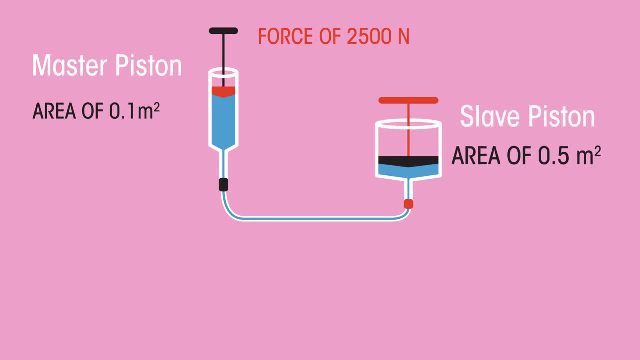 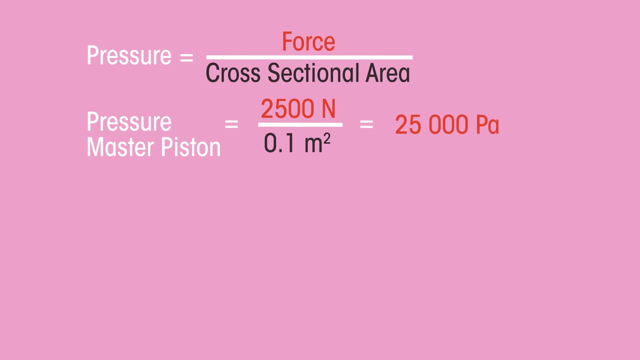 Calculate the force generated in the slave piston with a surface area of 0.5m2.. Pause the video and work it out. So the pressure produced by the master piston is 25,000 Pascals, and so the force produced by the slave piston is 25,000 times 0.5m2, giving 12,500 Newtons.